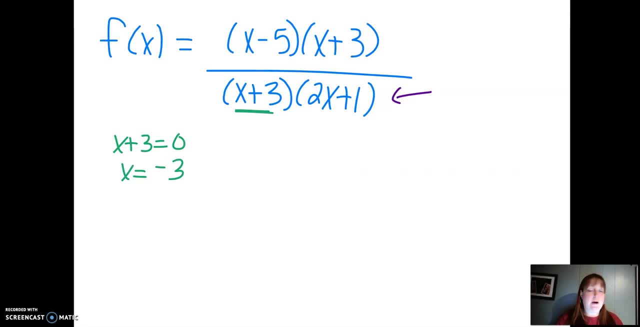 So we know that if I put in negative 3 right here I would get zero out. That would make the entire denominator zero. So I know that I have some type of discontinuity or some type of problem. I like to say at: x equals negative 3.. Then what about 2x plus 1? 2x plus 1 equals zero. 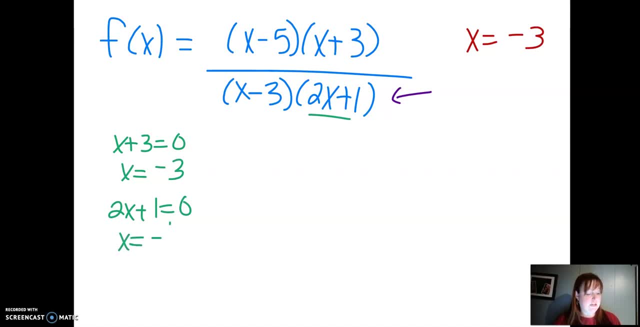 I subtract 1 from 1. Then I get x equals negative 1 half. That means again I have a problem or a discontinuity at x equals negative 1 half. That means the function doesn't exist at this point. 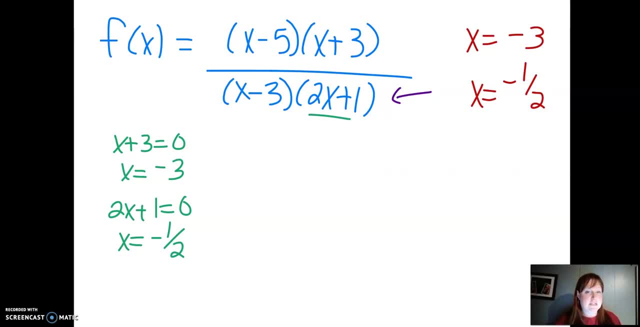 So those two points are my discontinuities. They're either going to be an asymptote or a whole. They're definitely one or the other. So I have to remember that's x plus 3.. So when I look at this I have to ask myself how do I know if it's a whole? 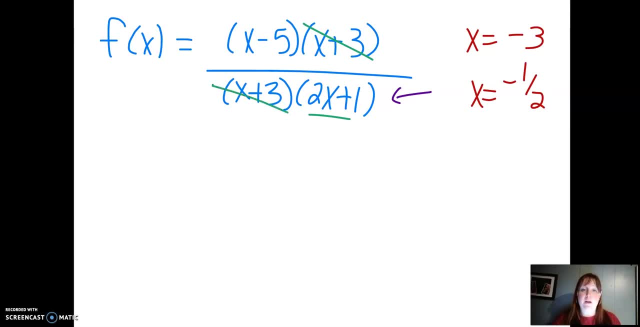 I notice that the top x plus 3, and x plus 3 on the bottom can cancel out. So what I know is that that's a whole okay. It cancels out and it simplifies to x minus 5 over 2x plus 1.. 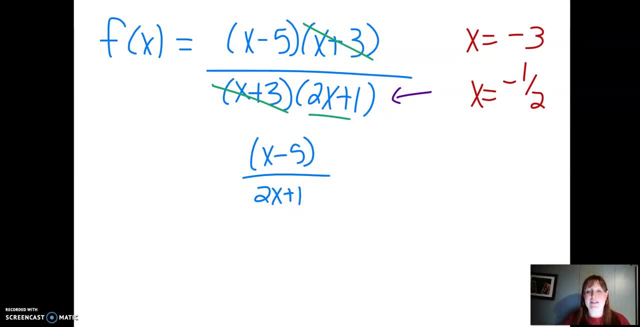 Now this top function and the bottom function look exactly the same. The only difference is this is going to have a whole at negative 3 and this one isn't. So that's how we know it's a whole. It canceled completely out, So we know there's a whole at negative 3, something We just 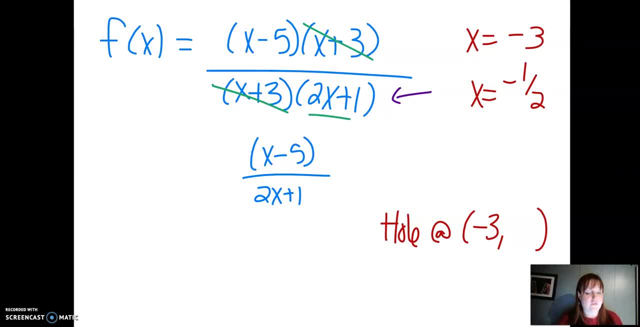 have to figure out what that something is because, remember, a whole is a point, It's a point on the graph. To figure out what that something is, we plug in negative 3 for x and we get negative 3 minus 5 over negative 6 plus 1, which is negative 8 over negative 5.. So we know we have a whole at. 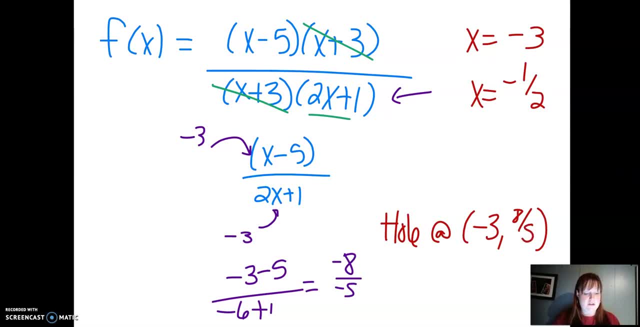 negative 3, 8 fifths. So that's a point on our graph. And then we know that since this 2x plus 1 did not cancel out, we have a vertical asymptote at x equals negative 1, half, and we can just write it like that, because 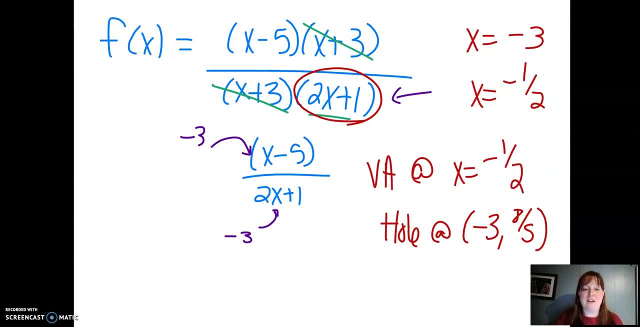 it's a line, It's just written like the equation of a line, So that's finding wholes and asymptotes.